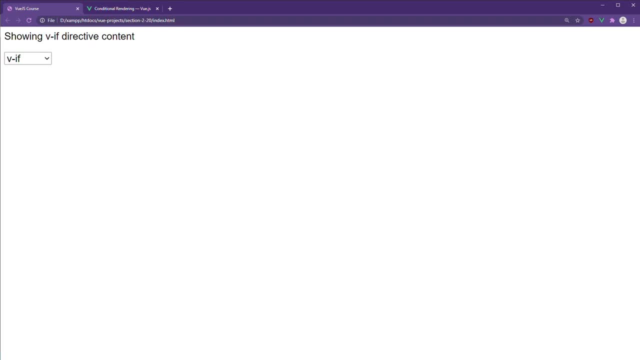 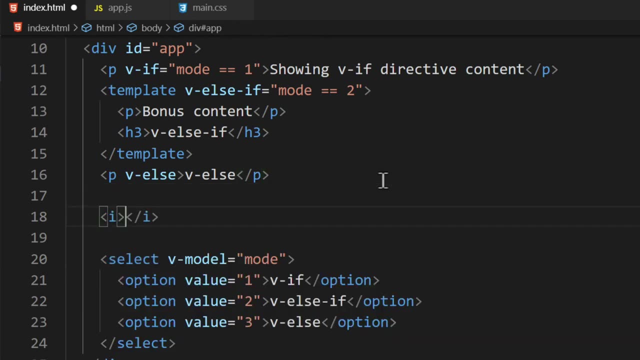 However, Vue provides a solution out of the box for this specific task. Back inside the template, we're going to add an Italics element with a simple message: We're going to apply the VShow directive. This directive expects a condition. We're going to set the condition to the following: Is Mode equal to 1.. 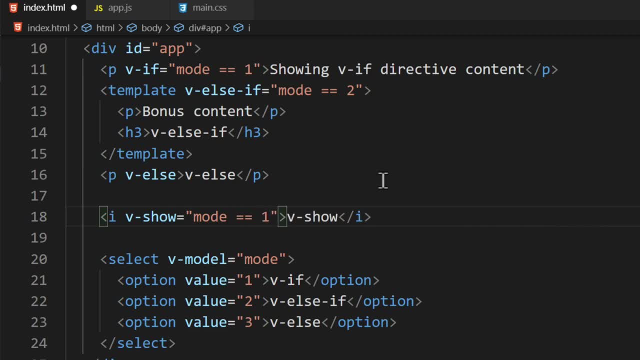 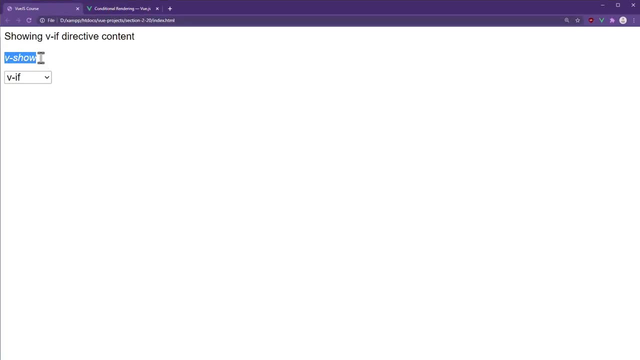 By default, the element should appear based on the condition. Let's give it a test. If I refresh the page, the element will appear without a problem. If I were to switch modes, it would disappear. It works similar to the VIF directives. 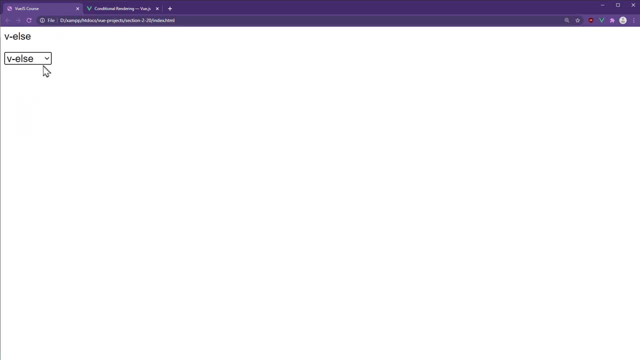 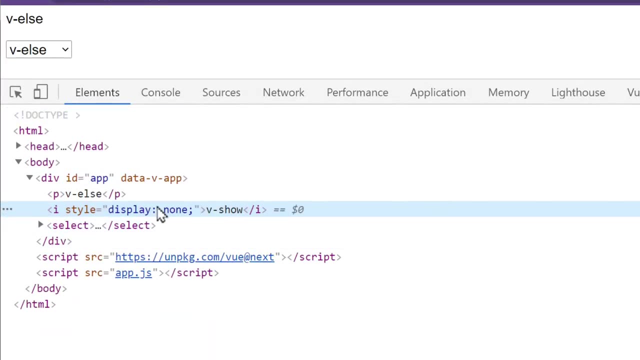 but with a different name. Vue will apply the Display CSS property. The value for this property will be None. This value hides the element from Vue. That's the main difference between VShow and VF directives. If I were to set the mode back to 1,, the silings are removed. 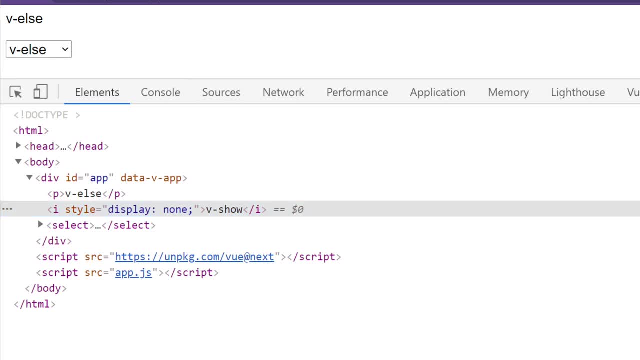 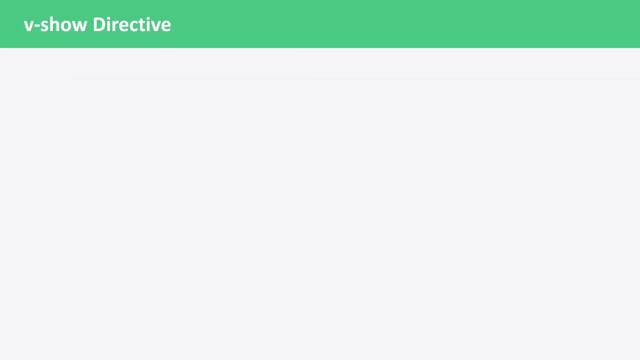 We've learned about the two ways to render elements in VF In this tutorial. we'll learn how to render elements in VF directly from the document. We'll also learn how to render elements in VF directly from the document. There are two ways to render elements conditionally. 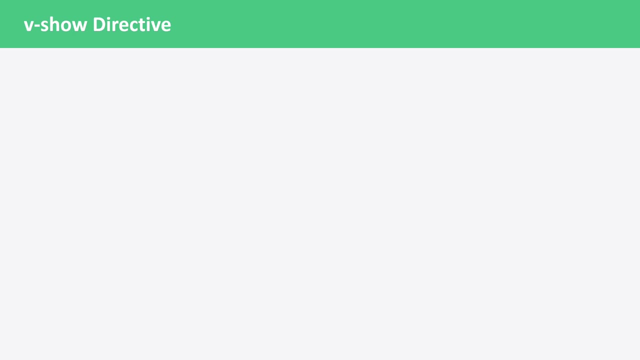 There are quite a considerable number of differences you should take into account whenever using them. Let's start with the VShow directive. Unlike the VIF directive, the element does not get removed if the condition turns out to be false. Instead, the element will remain in the document. The Display CSS property will be set to None. 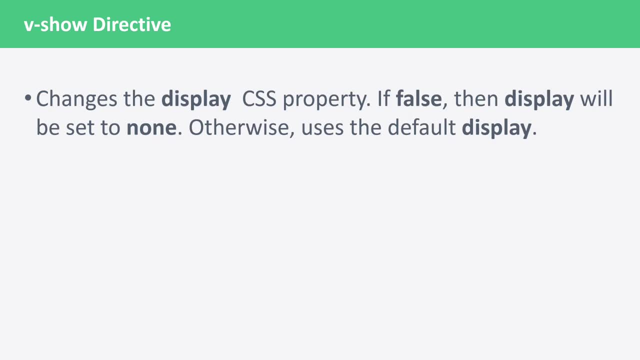 This value will hide it from Vue. You're limited to using the VShow directive alone. It will not work with the template tag I showed you, nor will it work with the VELSE directive. Something you should take into consideration is the performance you may gain or lose from using it. 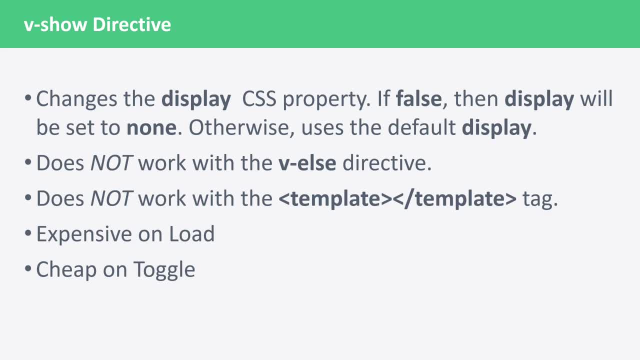 During the compilation of the template, Vue has to decide what has to be rendered. For every element added. you take a small performance hit. It isn't massive. It's not like your users will notice. However, it is a performance loss After the element is loaded, toggling the stylings of an